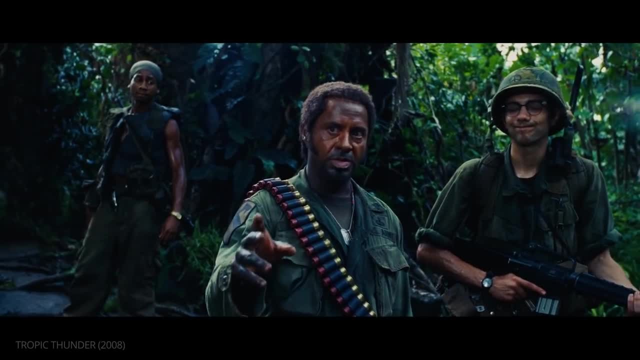 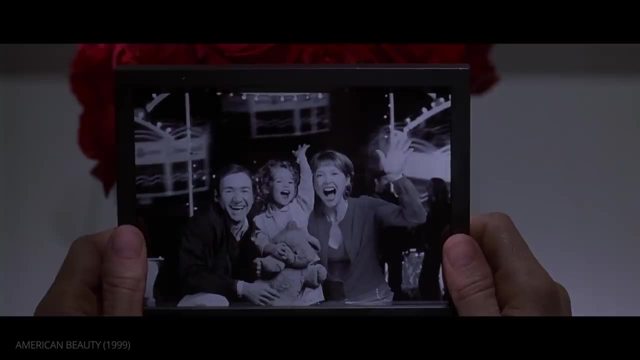 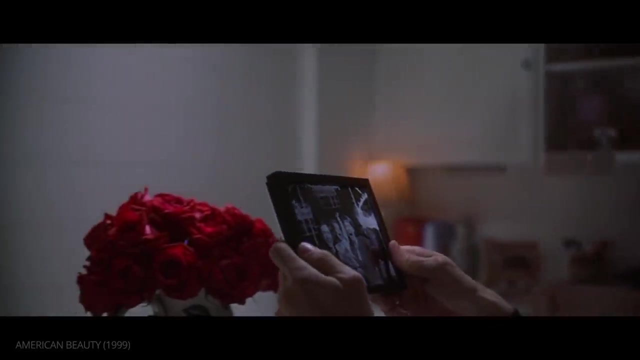 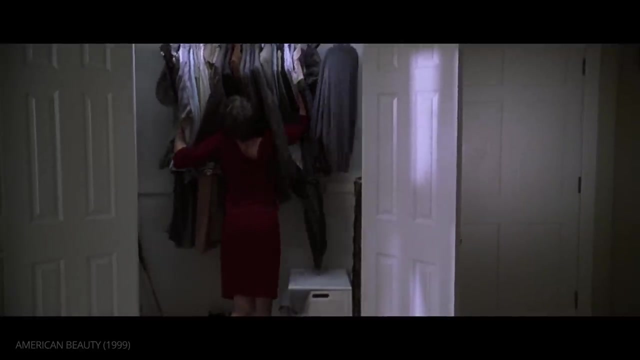 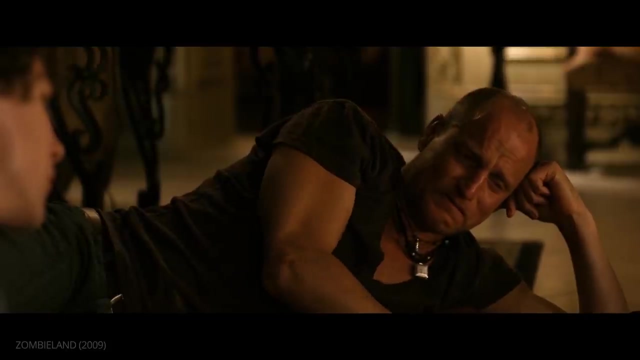 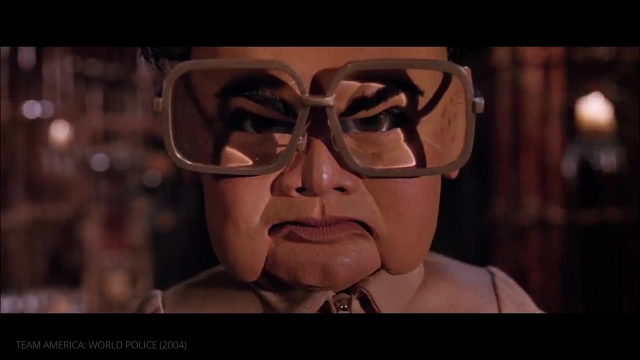 I don't believe you people. What do you mean you people? What do you mean you people? Or it can be heartbreaking- I haven't cried like that since Titanic. But there is one thing that is absolutely necessary in satire: A target. 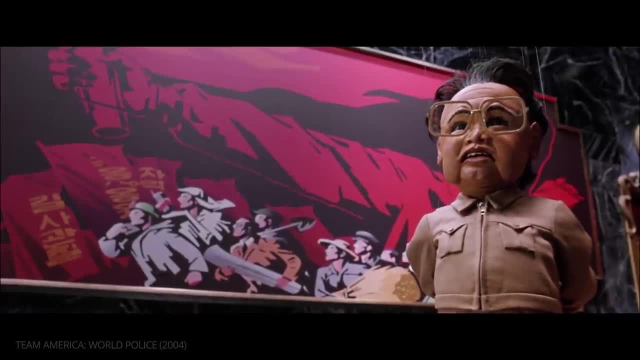 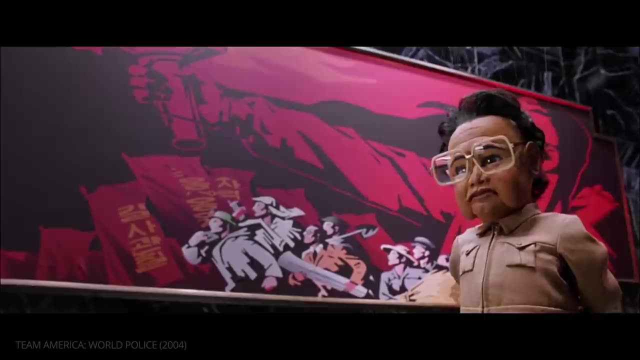 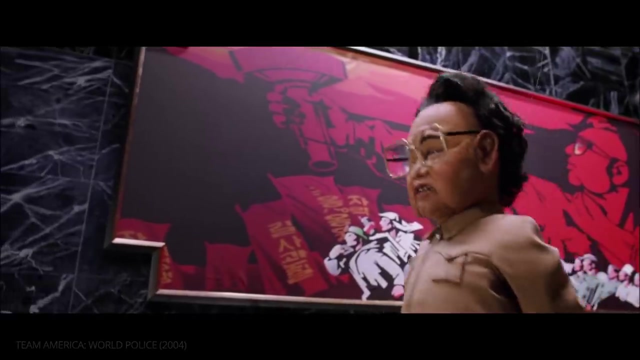 I'm so lonely, So lonely, So lonely inside real Rome. As long as there have been power structures, there have been satirists critiquing them Sitting on my little throne. Now let's go back to where it all started. 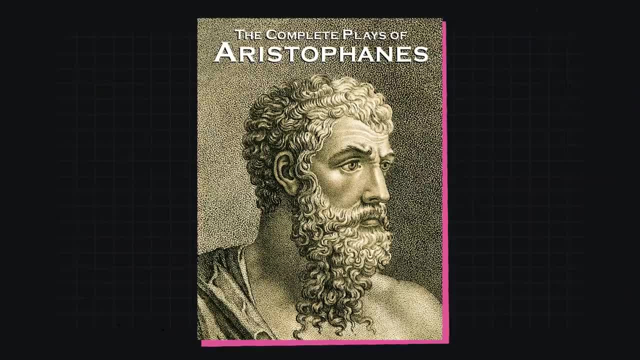 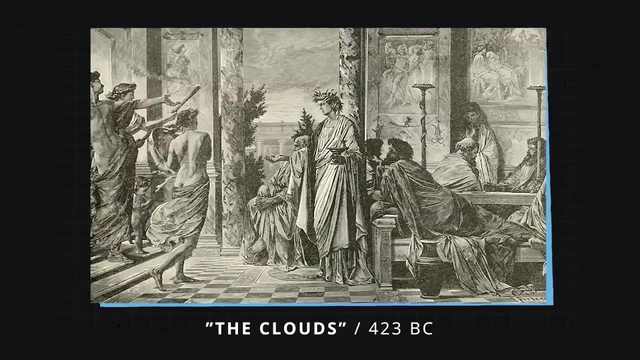 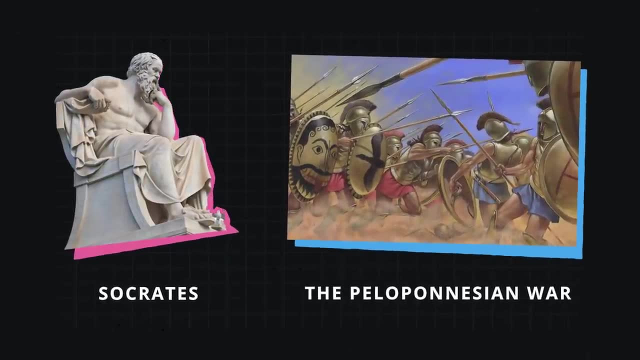 Ancient Greece and Rome. Most scholars point to a collection of plays written by Greek playwright Aristophanes as the earliest satire examples. These narratives used real people and situations of the era as the subjects of light and playful mockery. The original satire is the original. 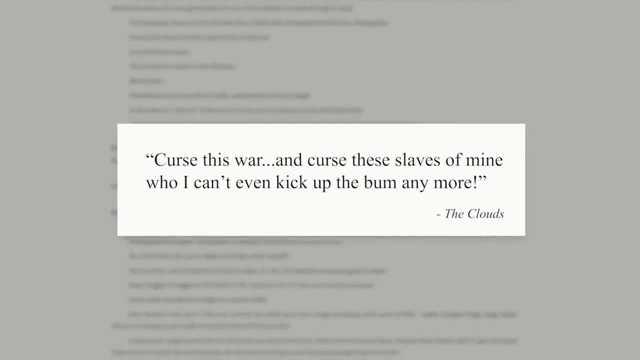 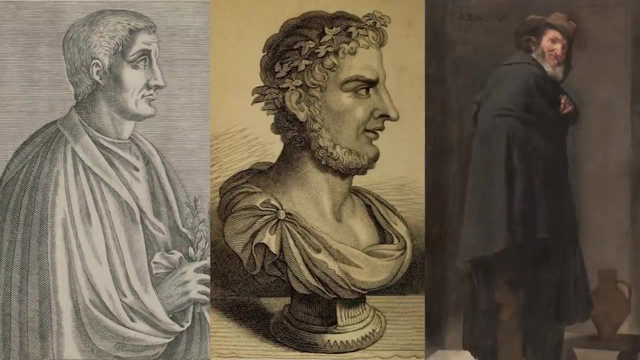 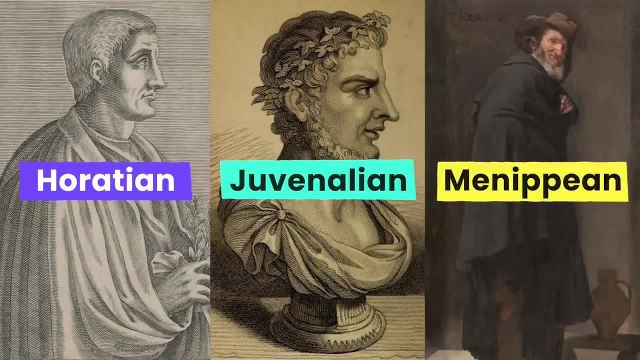 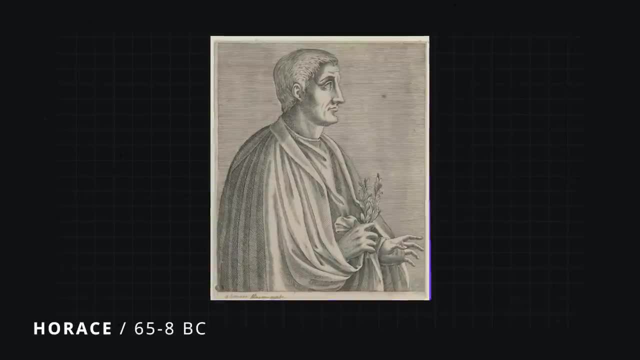 Horatian, Juvenalian and Menippean. Probably the most recognizable is Horatian satire, Named after the writer Horace, who was famous for his humorous ribbing of Roman society. Horatian satire, Horatian satire. 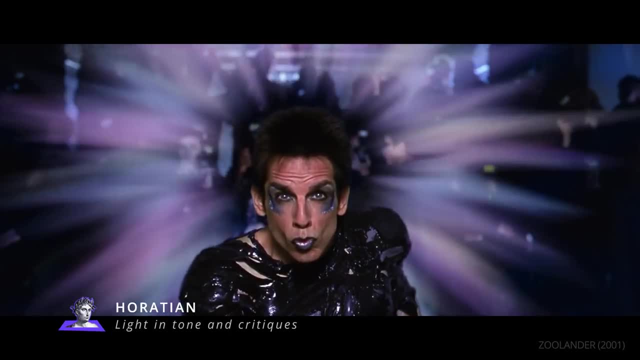 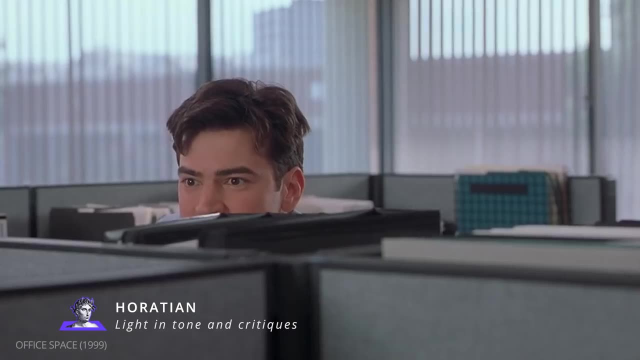 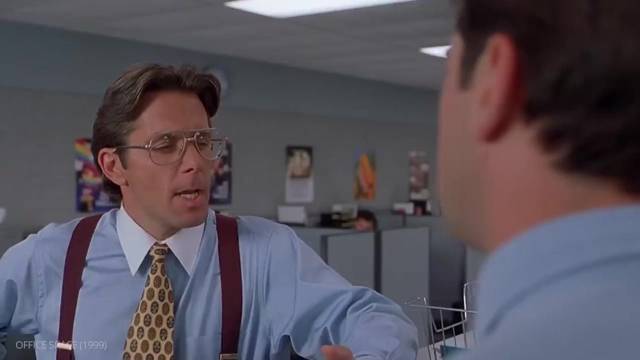 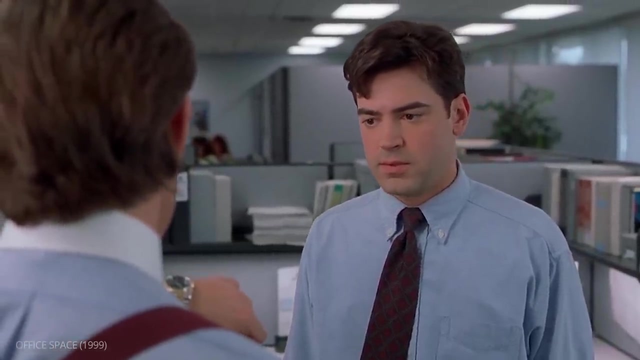 This type of satire is overtly comedic. Horatian satire: Light in tone and milder in its critiques. Horatian satire: Hello Peter, What's happening? I'm gonna need you to go ahead and come in tomorrow, So if you could be here around nine. 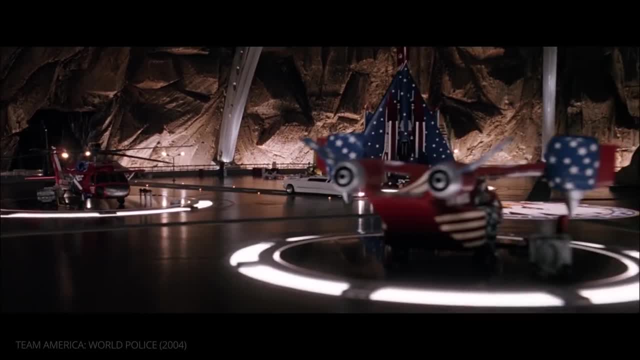 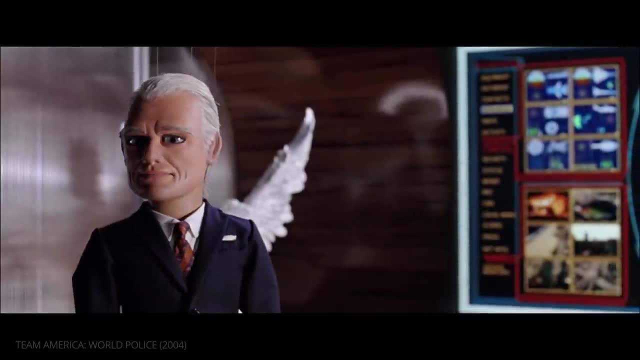 that would be great. Okay, Whether it be about American imperialism, We've been doing our best to keep the world safe, Gary. But now somebody has supplied the terrorists with WMDs And intelligence tells us they plan to use them. Isn't that right intelligence? 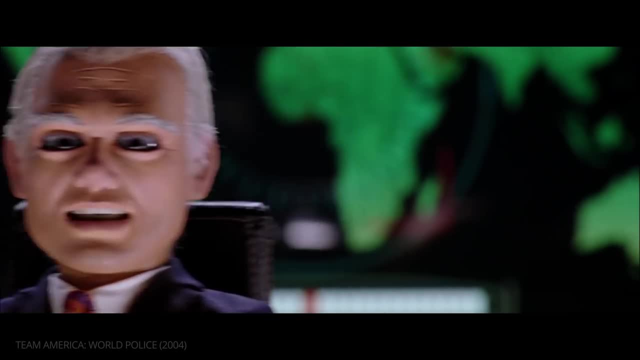 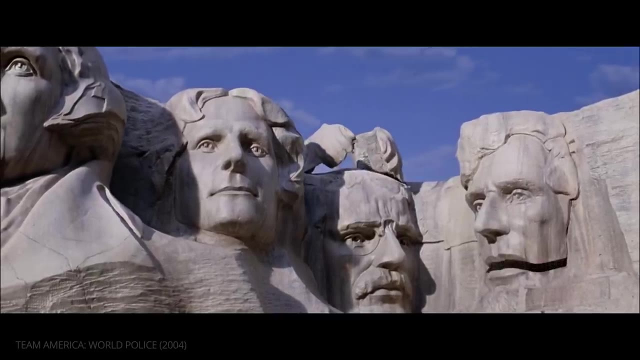 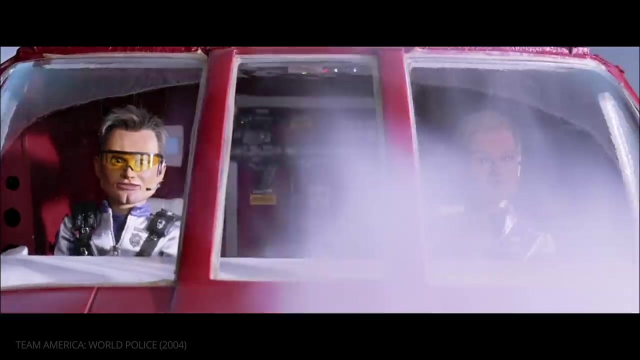 That is affirmative. All right, team. That's it. We've got a job to do. Let's go police the world. America, America, Yeah, Come at me again to save the world. Mother day, yeah. The fashion industry. 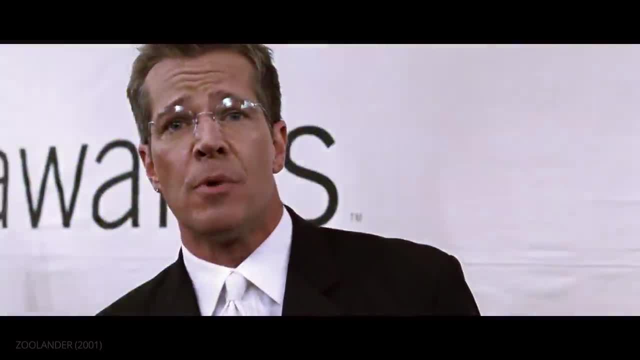 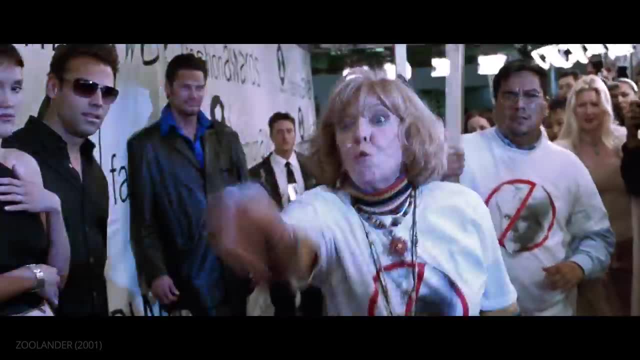 No denying: Jacobi Mugatu has been accused of exploiting cheap Malaysian workers to make his and most of the garment industry's clothes. Mugatu, screw you and your little dog chump. Look out, she's got an egg. Modern politics. 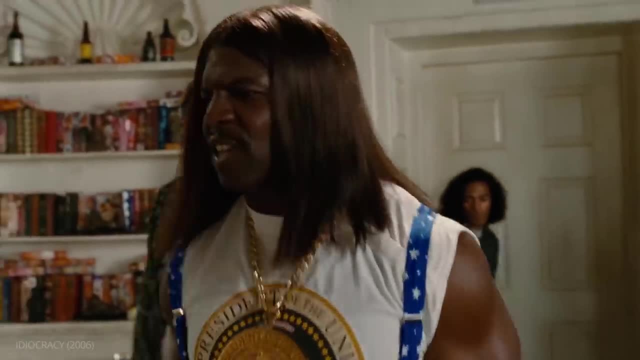 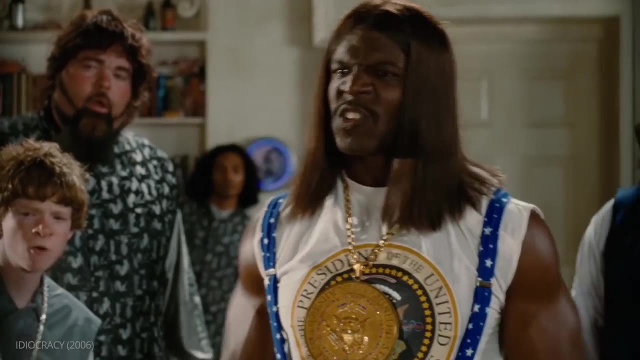 Dwayne Elizondo Camacho, five-time ultimate SmackDown champion and president of the United States, had called a special summit with the smartest man in the world. So you smart huh? No, I thought your hair would be bigger. 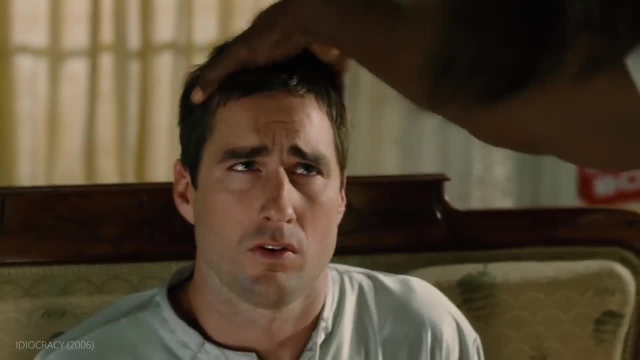 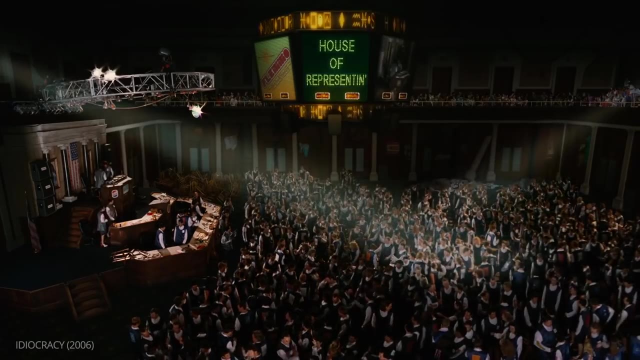 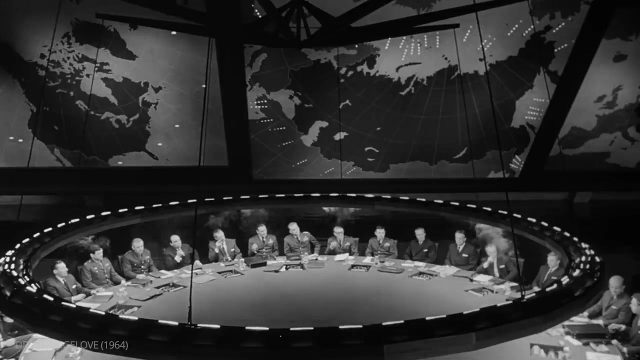 They won't make you angry about a particular subject, but after all the laughter they'll make you think. Let's get you sworn in. Dr Strangelove was released in 1964, at the heart of the Cold War, And it's a great example of a satire tackling a dominant political issue of the era. 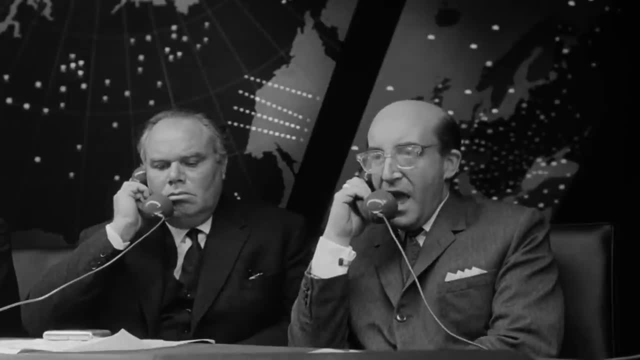 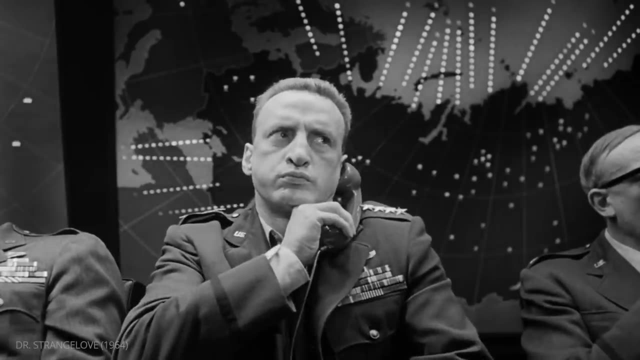 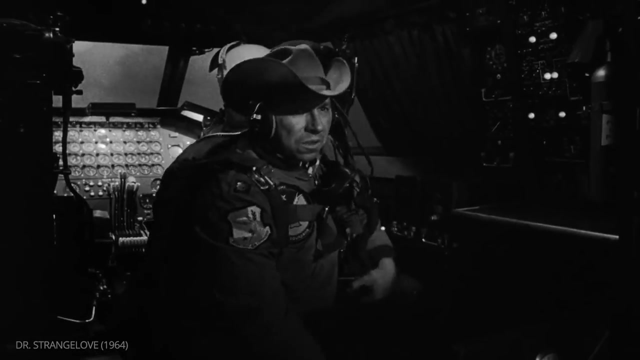 nuclear brinkmanship, Dr Strangelove. Now then, Dimitri, you know how we've always talked about the bomb, the hydrogen bomb. Well, boys, I reckon this is it: Nuclear combat, toe-to-toe with the Ruskies. 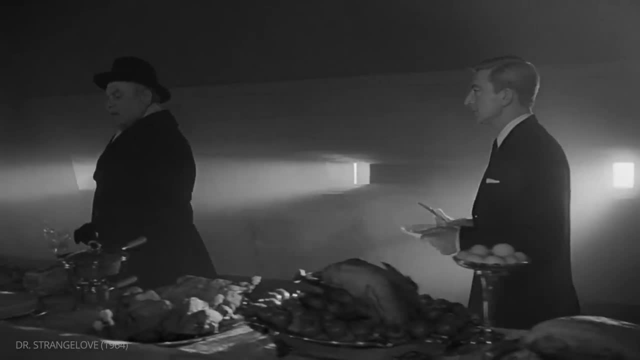 Irony is laced throughout the dialogue. And bring me some cigars, please, Havana cigars. And that will be all for you soon. Yes, And I'll see to it right away. Try one more time. Try one of these Jamaican cigars, Ambassador. 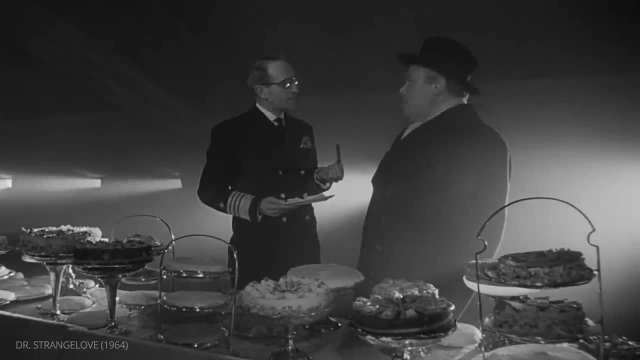 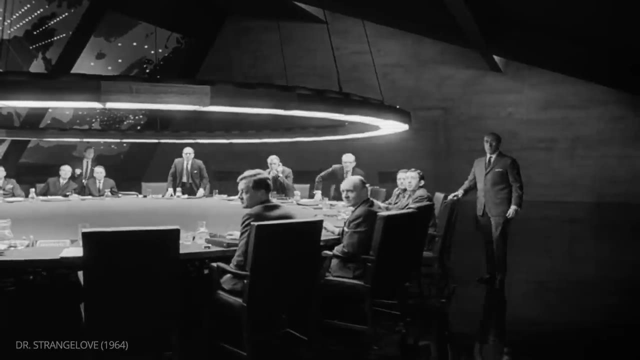 They're pretty good, Thank you. no, I do not support the work of imperialist stooges. Oh only commie stooges huh And highlights how oblivious these men are to the power they wield. But the whole point of the doomsday machine is lost. 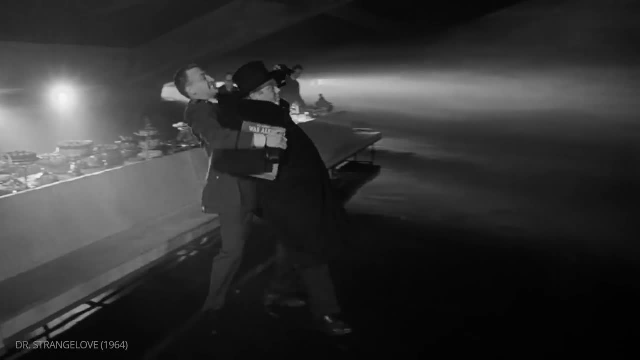 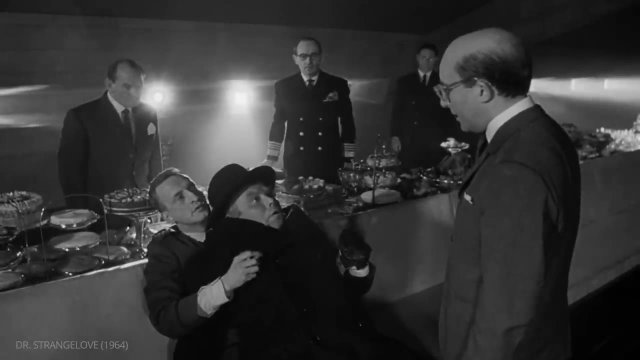 If you keep it a secret, why didn't you tell the world? eh, And the consequences of failure. Gentlemen, you can't fight in here. This is the war room. No, fighting in the war room. Haha, that's rich. 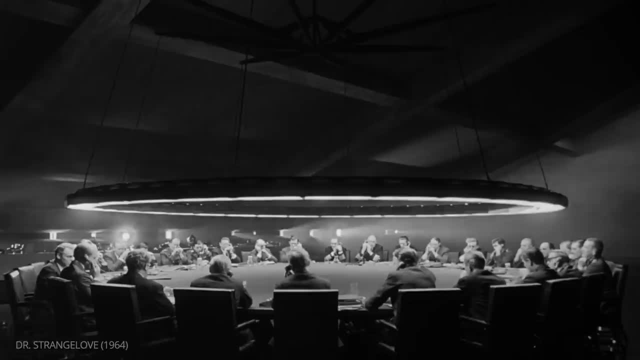 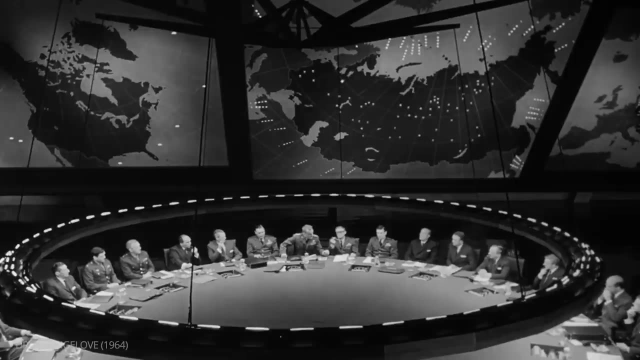 And the war room itself is a great example of satirical exaggeration Which is comically massive and extravagant, clearly illustrating the military-industrial complex: bloat. If the pilot's good see, I mean if he's really sharp- he can barrel that baby in solo. 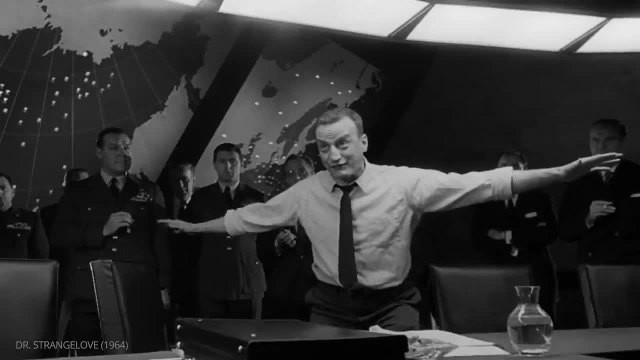 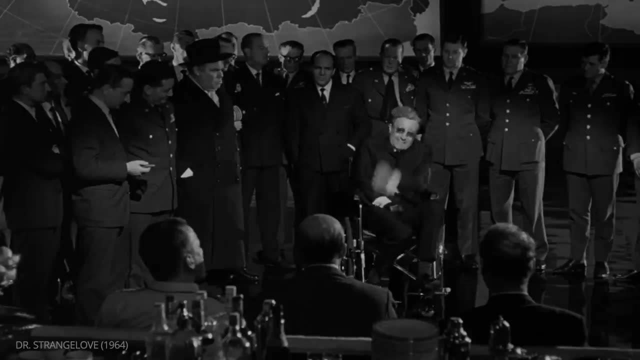 I mean you ought to see it sometime. It's a sight, a big plane like a 52. Vroom, It's jet exhaust, flying tickets in the barnyard. All these techniques make Dr Strangelove a quintessential Horatian satire. 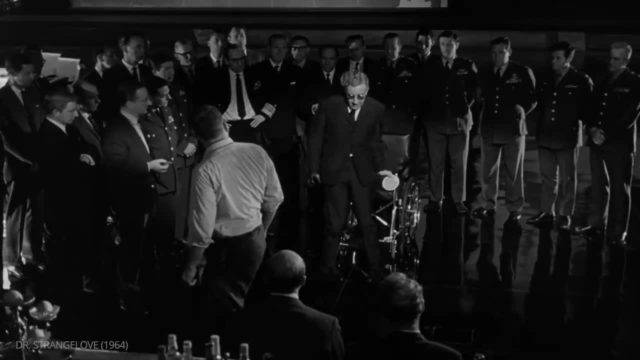 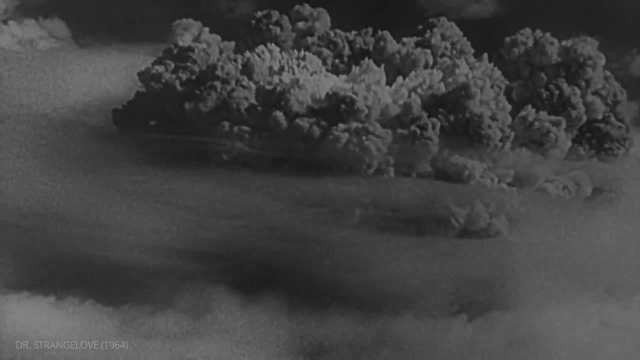 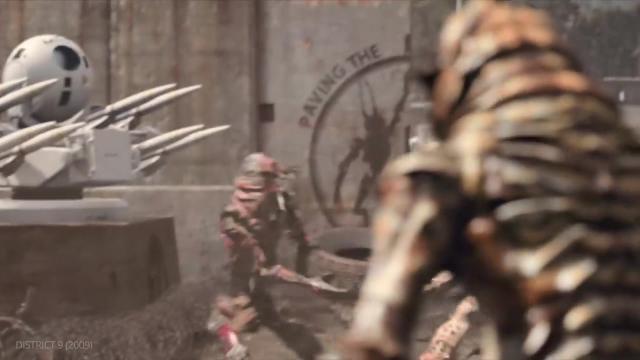 "- Monsieur Hasn't walked", A gut-busting comedy that lampoons the absurdity of nuclear war. "- Meet her again". Now what if, instead of making the audience laugh, we want to make them angry? Enter Juvenalian satire. 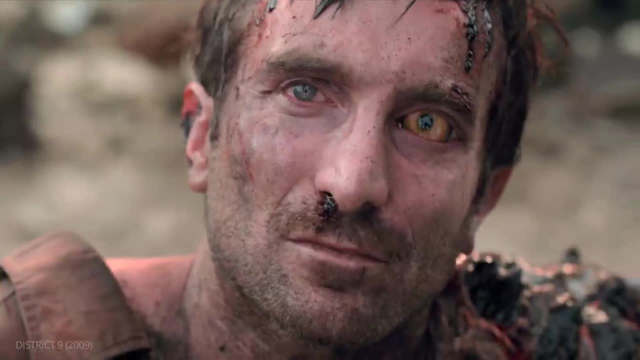 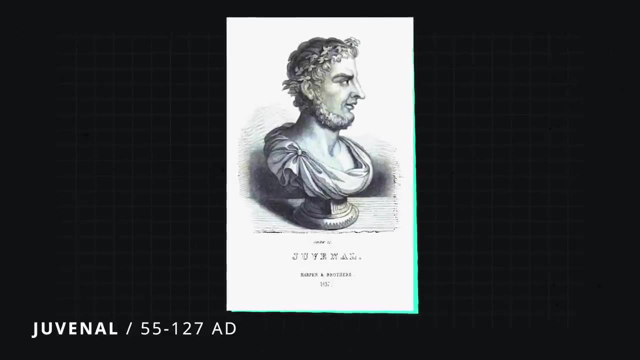 Horatian's darker and more cynical counterpart. It's named after Juvenal, a writer known for his abrasive and vicious rhetorical attacks on Roman elites and power structures. It can still be funny, but it is often more derisive and rooted in drama. 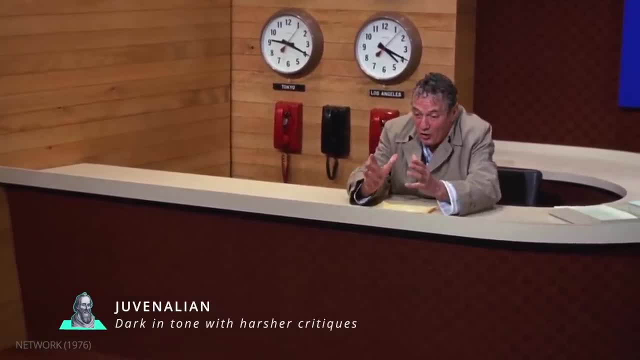 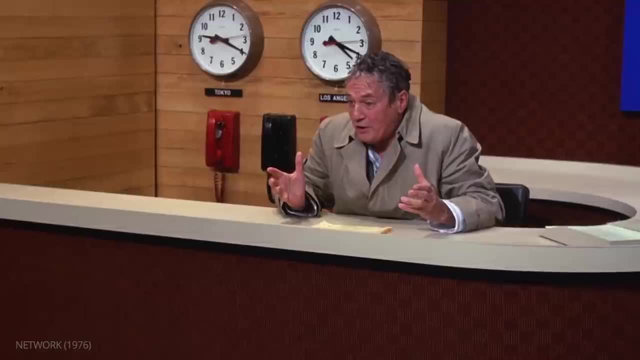 "- So we don't go out anymore, We sit in the house and slowly the world we're living in is getting smaller and all we say is: please at least leave us alone in our living rooms, Let me have my toaster and my TV and my steel-belted radios. 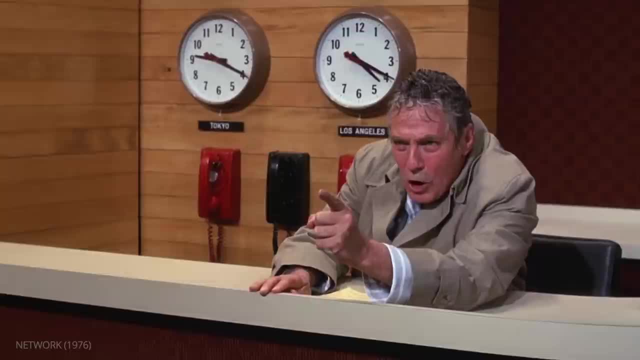 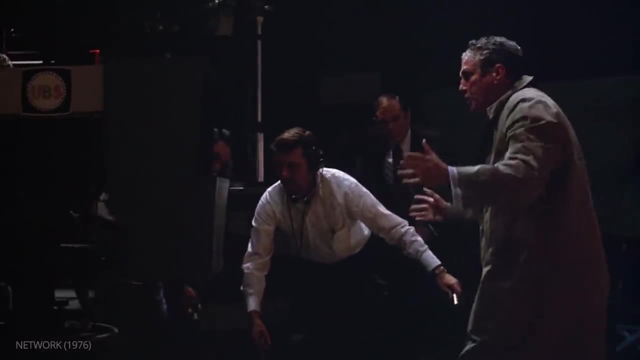 and I won't say anything. Just leave us alone. Well, I'm not going to leave you alone. I want you to get mad". "-. Then we'll figure out what to do about the depression and the inflation and the oil crisis, But first get up out of your chairs, open the window. 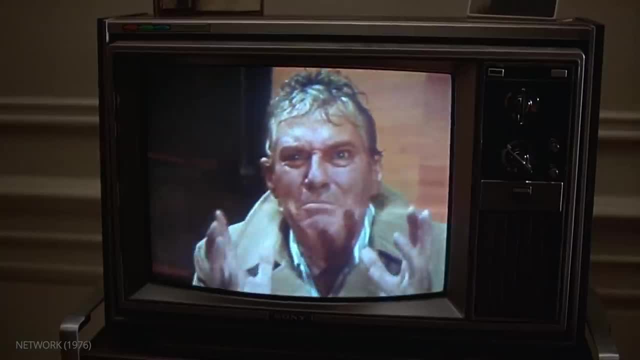 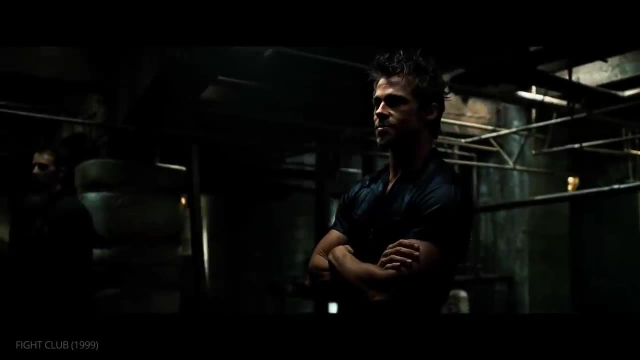 stick your head out and yell and say: I'm as mad as hell and I'm not going to take this anymore". Welcome to Fight Club. Think of Fight Club. The first rule of Fight Club is: you do not talk about Fight Club. 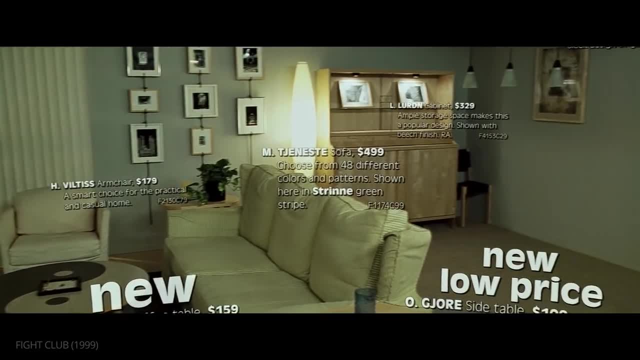 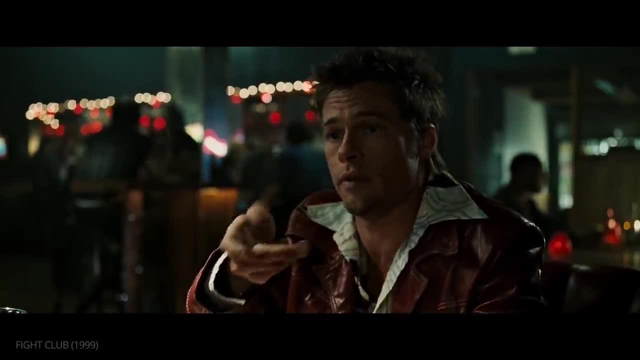 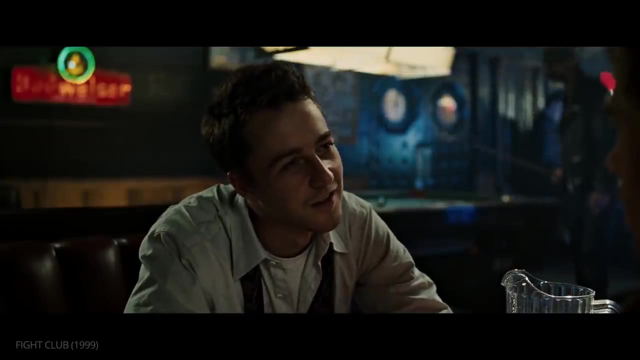 A Juvenalian satire, of course, Consumer culture "-. We are consumers, We are byproducts of a lifestyle obsession Or celebrity magazines, Television with 500 channels, Some guy's name on my underwear, Rogaine Viagra, I say never be complete. 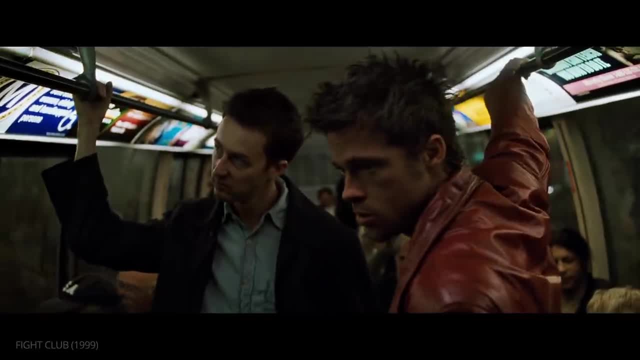 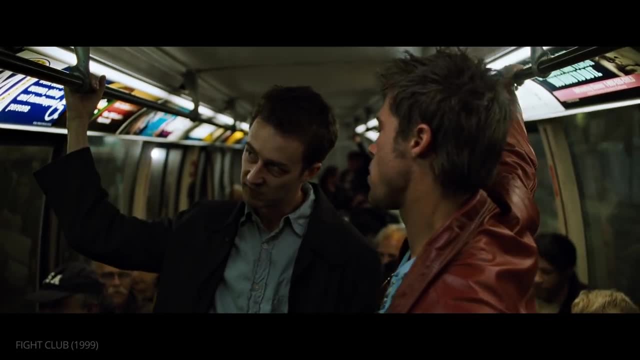 I say: stop being perfect" And toxic masculinity "-. I felt sorry for guys packed into gyms trying to look like how Calvin Klein or Tommy Hilfiger said they should". We can also look at Neil Blomkamp's District 9.. 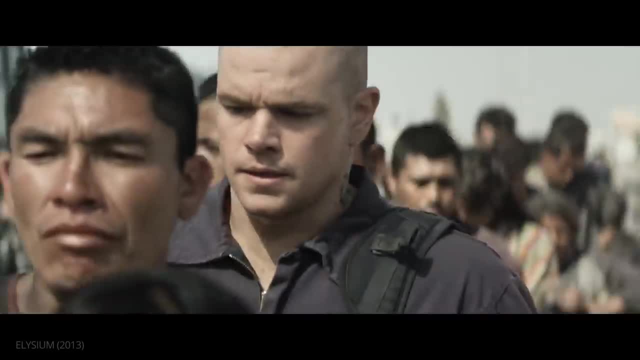 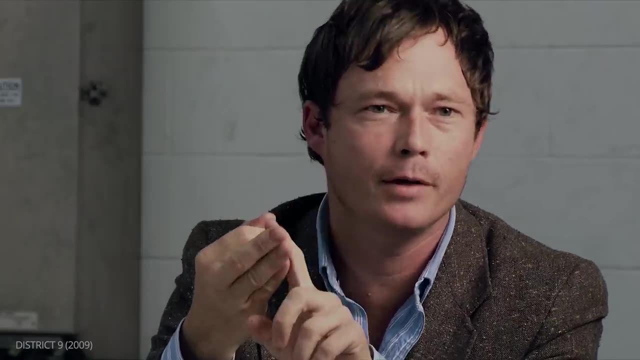 And Elysium, Both of which tackle racial and economic inequality "-. The creatures were extremely malnourished, They were very unhealthy, They seemed to be aimless. There was a lot of international pressure on us at the time And the entire world was looking at Johannesburg. 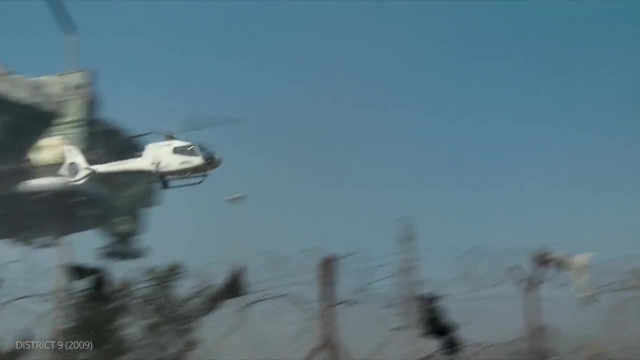 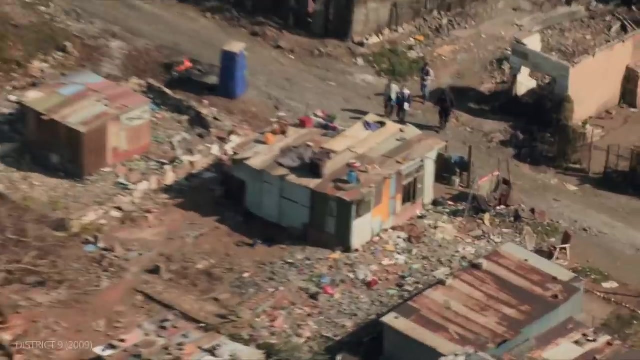 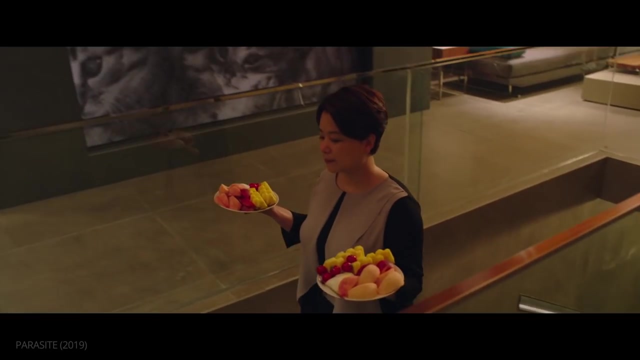 So we had to do the right thing". "- What was a temporary holding zone soon became fenced, became militarized, And before we knew it, it was a slum". One of the most celebrated juvenalian satires in recent years is Bong Joon-ho's Parasite. 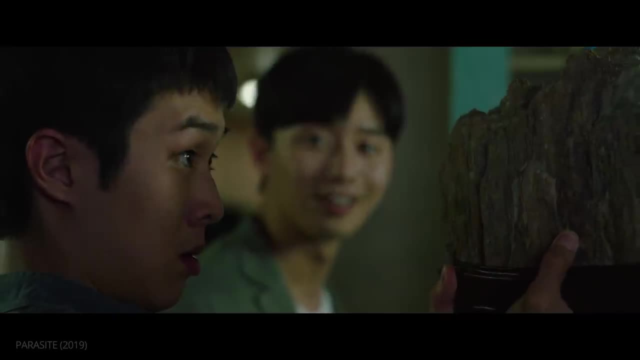 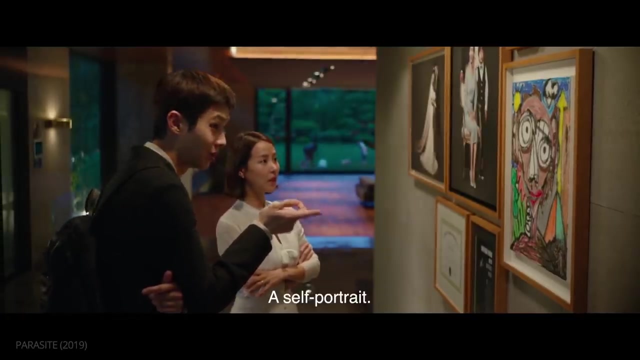 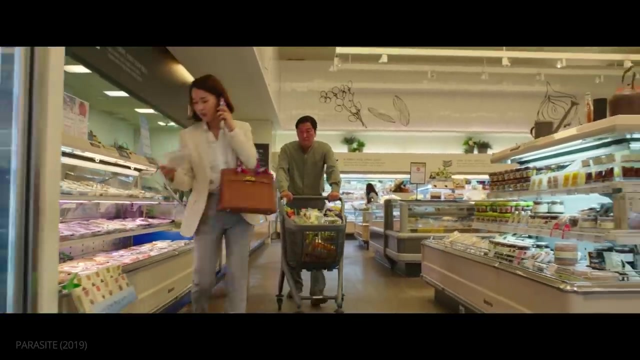 "- Wow, this is really symbolic". Of course there are jokes in Parasite: "- Our Dasong is totally artistic. Look at this". "- Did you draw a chimpanzee". "- It's a self-portrait". "- As expected". But the real satire of the film lies in its straight-faced depiction of the vast gulf. 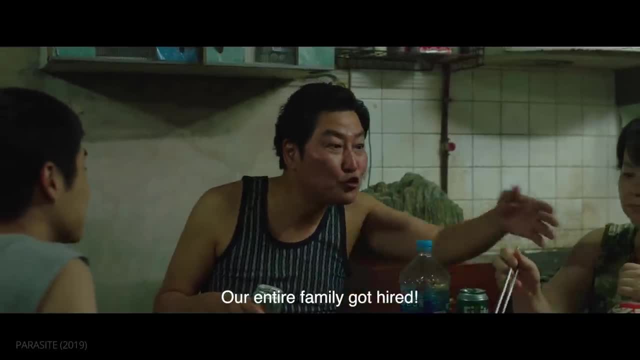 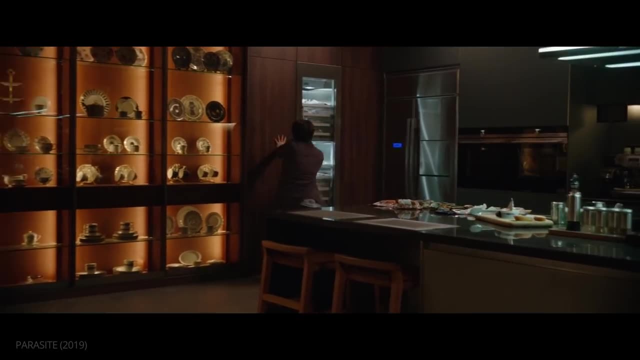 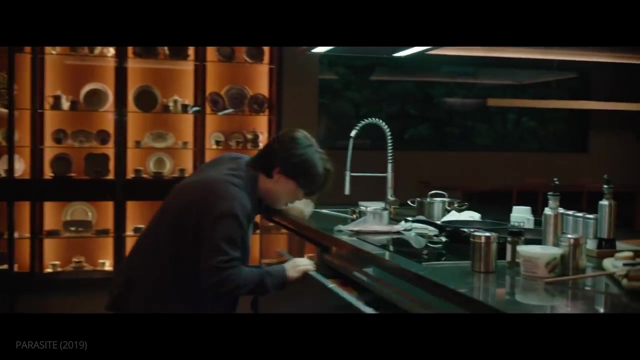 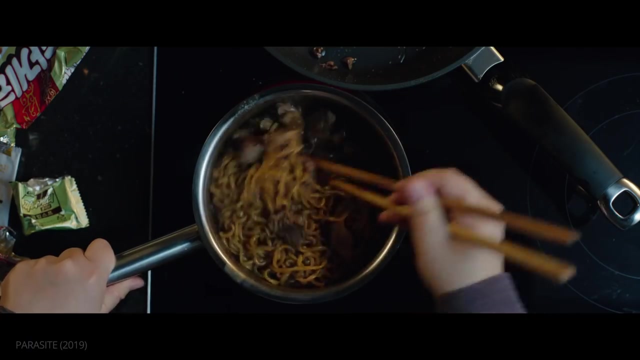 between the haves And have-nots "-. We can see irony in the noodle dish prepared by Moon Gwang, A dish using instant noodles topped with expensive beef, A symbol for the collision between rich and poor which lays at the heart of Parasite's message. 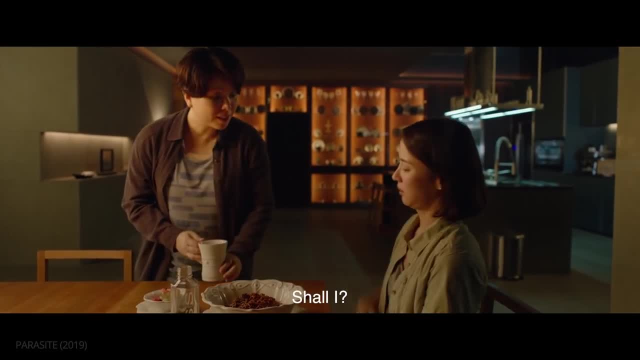 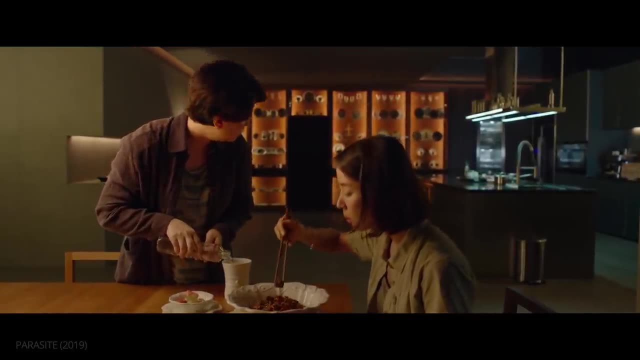 "- You're just like an old lady when it comes to jjapaguri". "- You think so? Oh no, You can tell me to eat Dasong's food. The sky is dirty here too, Huh. "- Dahye. 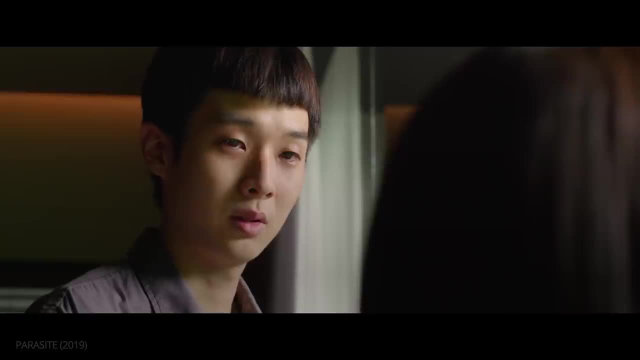 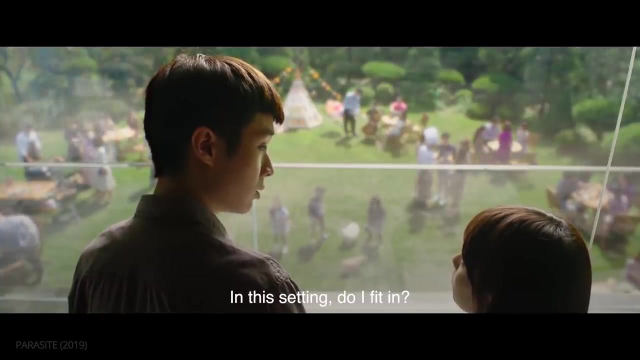 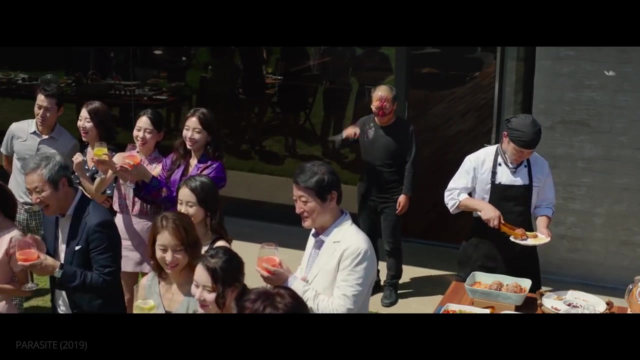 Huh, Do I look good in it? "-. What do you think, Do I look good in it Here? At times it's heartbreaking And then it's disturbing, It's nerve-racking, But Can't really lie, I've never lived that way". 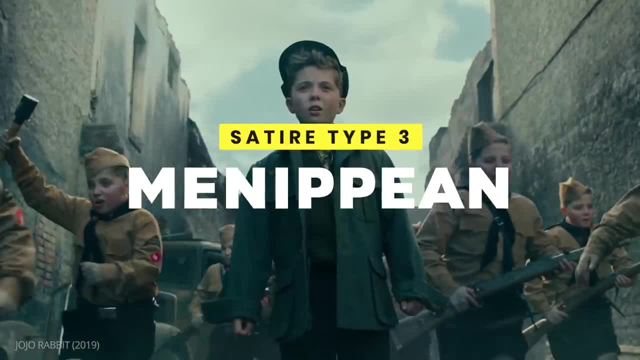 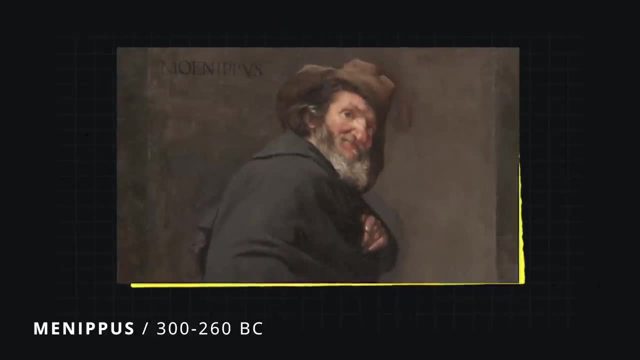 And finally "- Okay, come here. Okay, See that American there, Just go give him a hug, Go run, Let's go. Our final form of satire is, and mannipian Little is known about the Greek-writer Manippus. 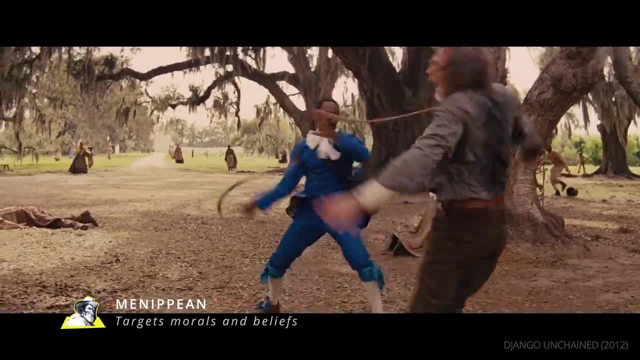 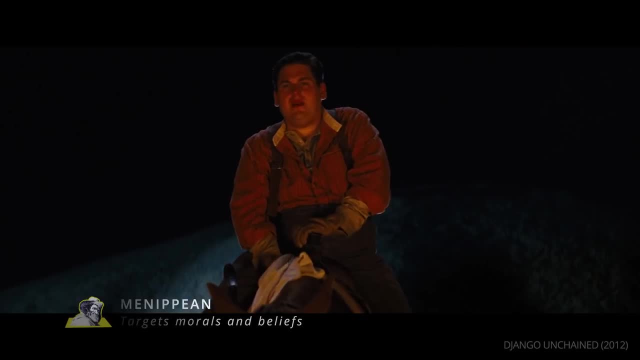 because all of his work has been lost to time, or moral attitude. That attitude can be racism: "- Damn, I can't see fucking shit out of this thing". "- Anybody bring any extra bags". Greed, "- Was all this legal? 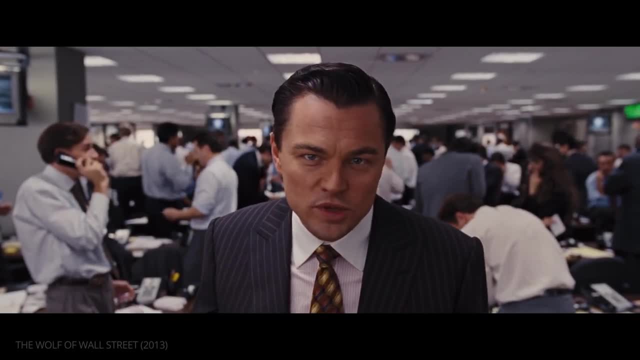 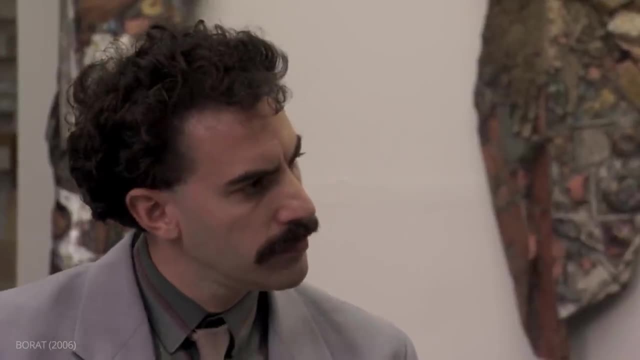 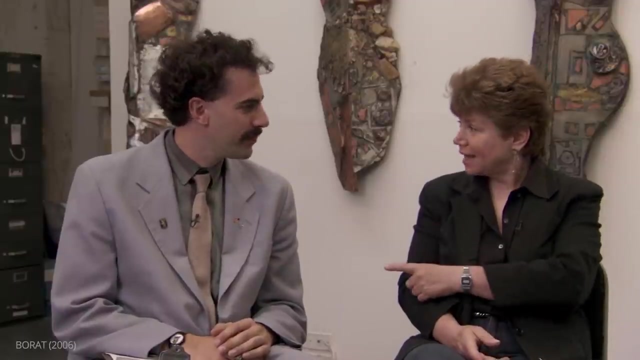 Absolutely fucking not, But we were making more money than we knew what to do with" Sexism "- So what? that means that this is feminism". "- It's the theory that women should be equal to men in matters economic, social and political". 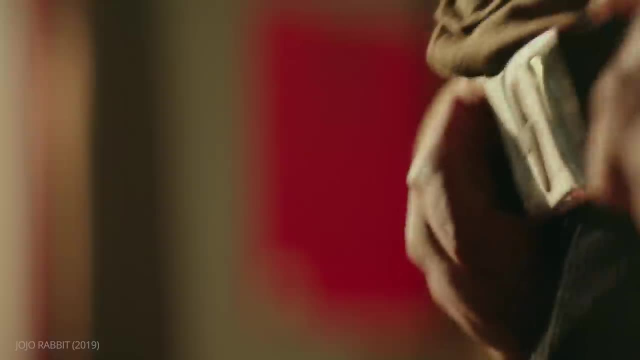 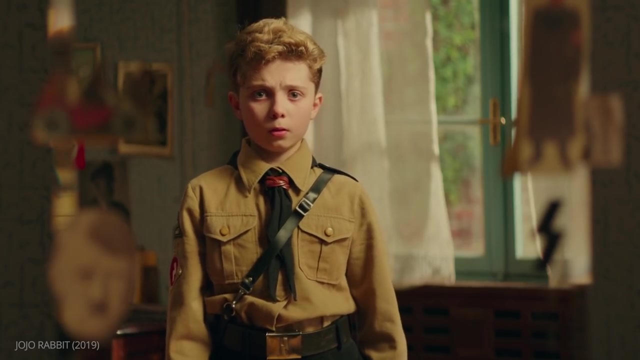 "- Now you are laughing. That is the problem". Anything the filmmaker deems to be morally repugnant. "- Jojo Betzler, 10 years old". Jojo Rabbit is a Manipian satire which has a pretty clear target: fascism. 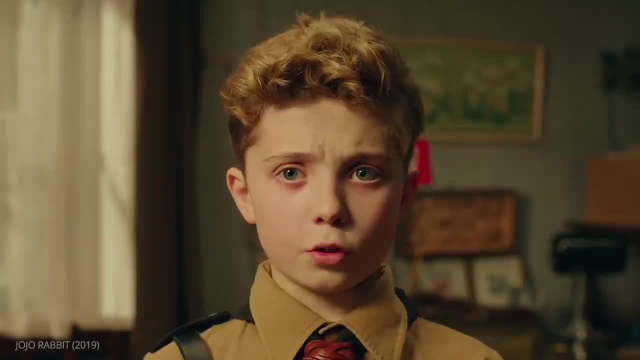 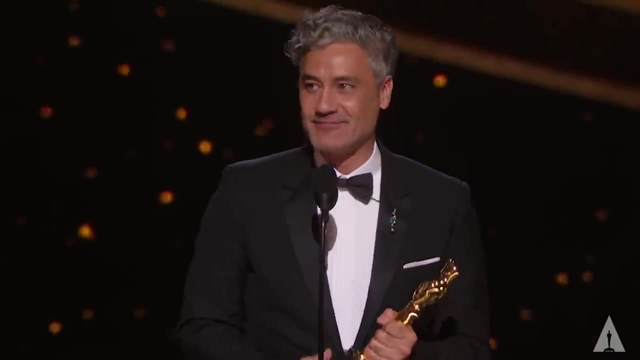 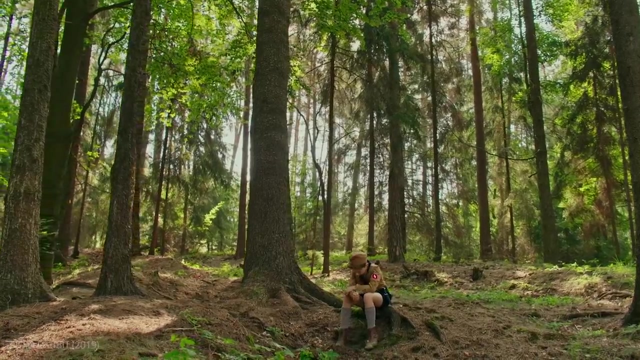 "- I swear to devote all my energies and my strength to the savior of our country, Adolf Hitler". Writer-director Taika Waititi adapted Caging Skies, a novel with a darker and more serious tone, and added his own comic sensibilities. 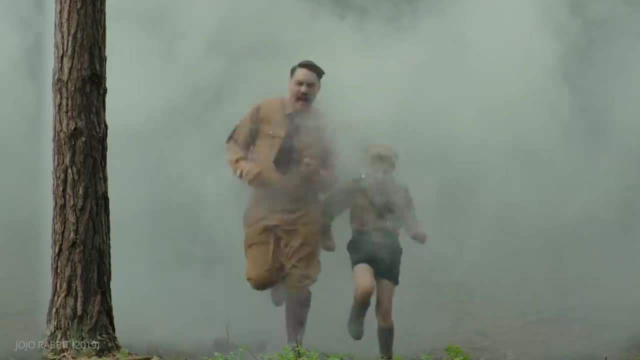 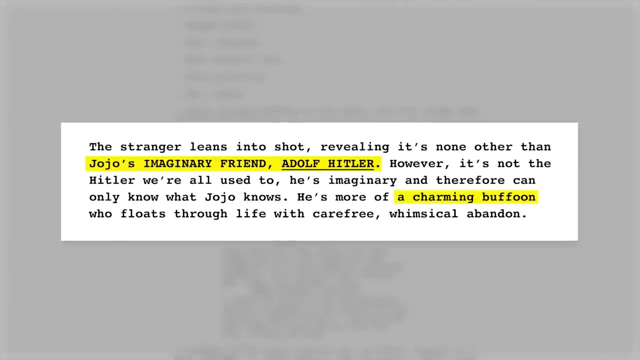 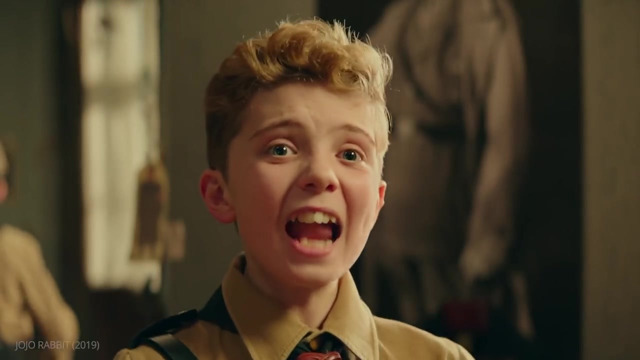 to create a satire that is both tragic and hilarious. Consider the presentation of Hitler as Jojo's imaginary friend in the script. He's a charming buffoon who floats through life with carefree, whimsical abandon By depicting a cartoonish, exaggerated Hitler. 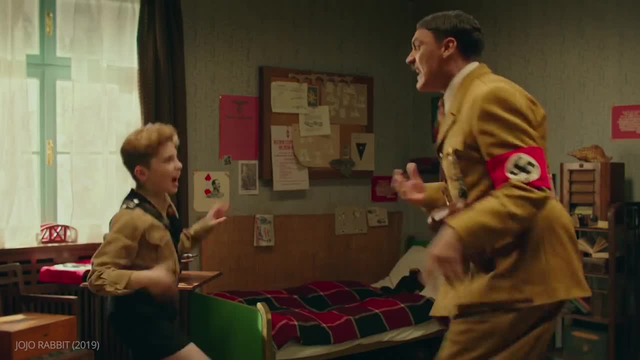 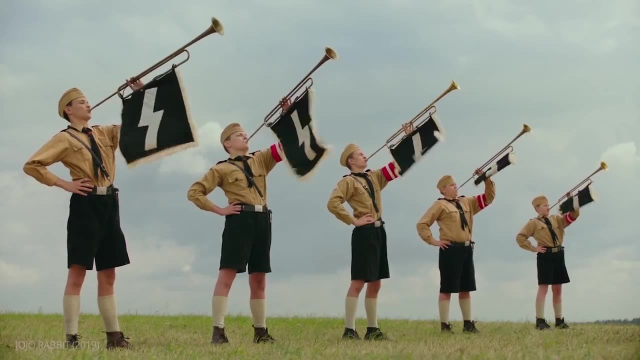 "- You're gonna be the best, Hitler, Hitler, You can do it. Hitler, Hitler, Hitler, Hitler, Hitler, Hitler. Why? TT heightens the absurdity of fascistic beliefs, Like this ludicrous biology lesson "- Fangs. 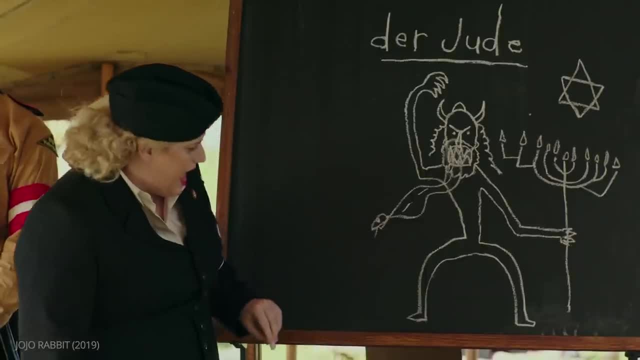 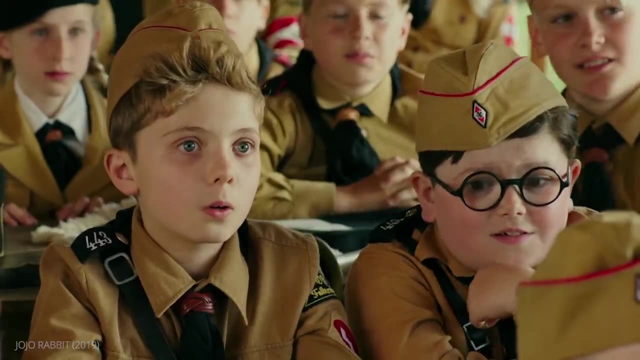 Fangs Yuck Serpent's tongue. Serpent's tongue Steals Yuck Scales, Because once upon a time a Jewish man mated with a fish. We Aryans are 1,000 times more civilized and advanced. 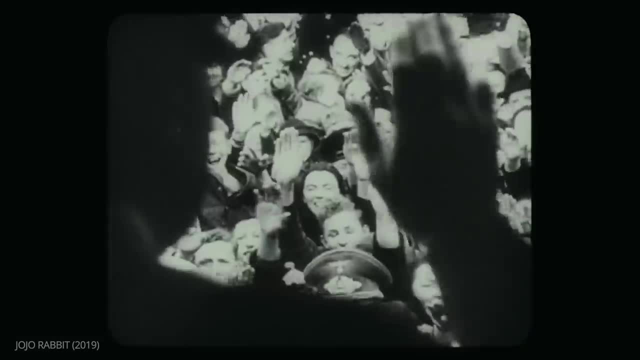 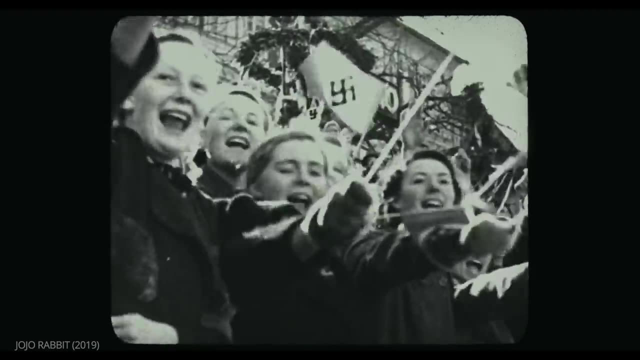 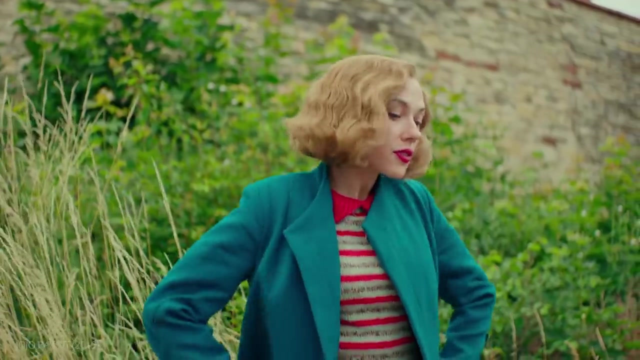 than any other race. Irony is also on full display in JoJo, using a German cover of I Wanna Hold Your Hand. during the opening credits, The rather vibrant and unexpected color palette: "- Dancing for people who don't have a job. Dancing for people who are free. 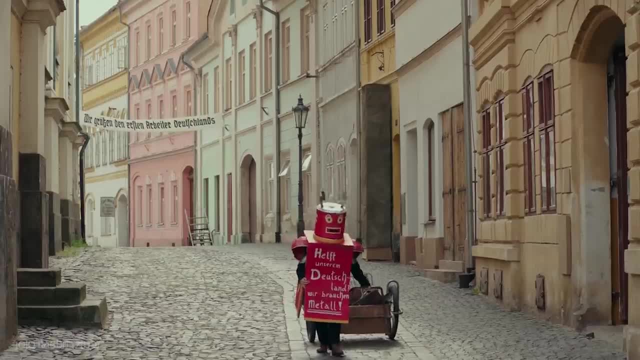 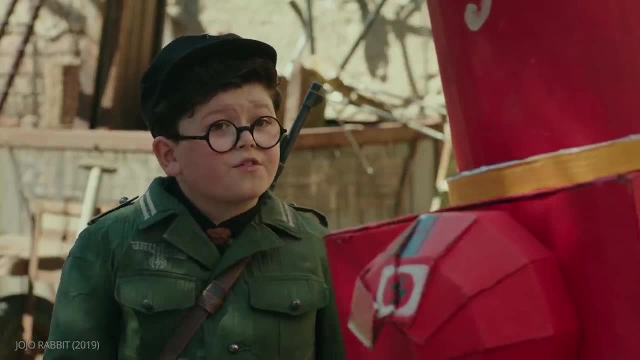 It's an escape from all this" And the absurd delusion of propaganda. "-. I caught a Jew, A real one, Oh, a Jew. I saw some that they caught hiding in the forest last month. Personally, I didn't see what all the fuss was about. 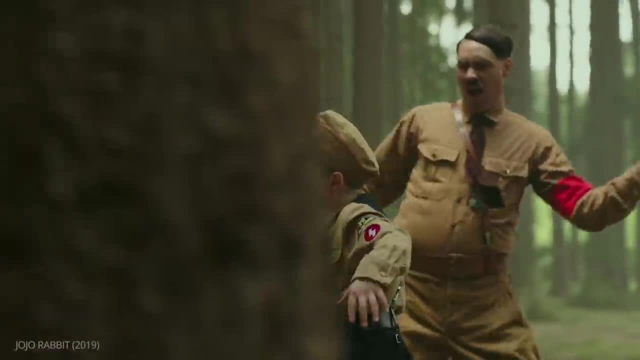 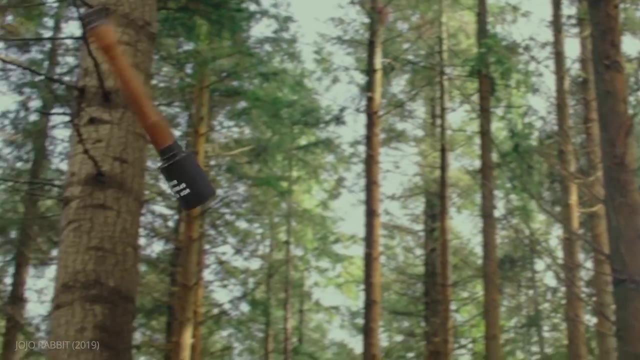 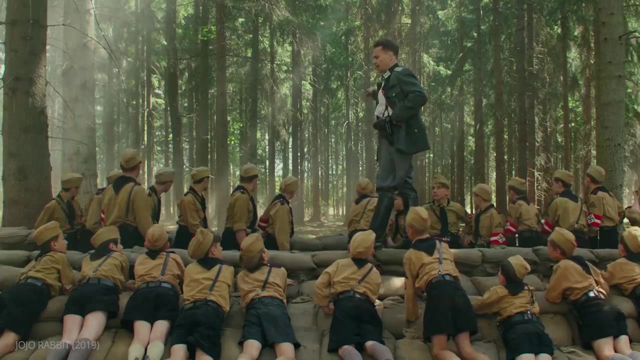 They weren't at all scary and seemed kind of normal". The tone of Jojo Rabbit is indicative of the wide range of tone a Manipian satire can take. It can be anything from slapstick "- Don't do that" to tragedy. 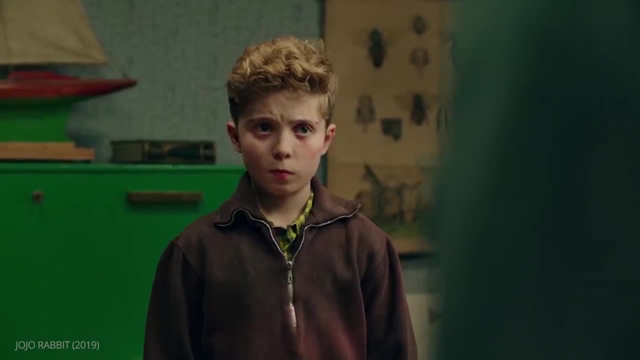 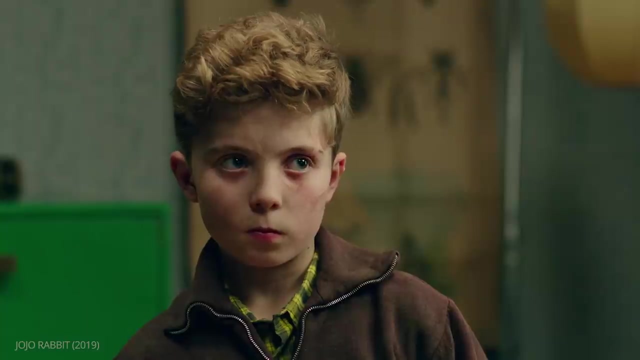 It's all Manipian, as long as its target is a belief or moral attitude "-. You're gonna put this on, okay, You're gonna forget about that disgusting dewy cow up there and you're gonna come back to me, where you belong. 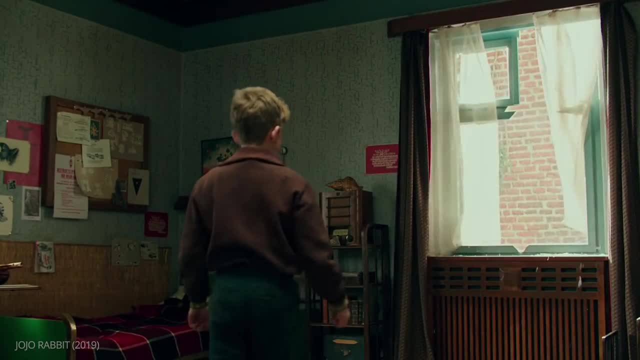 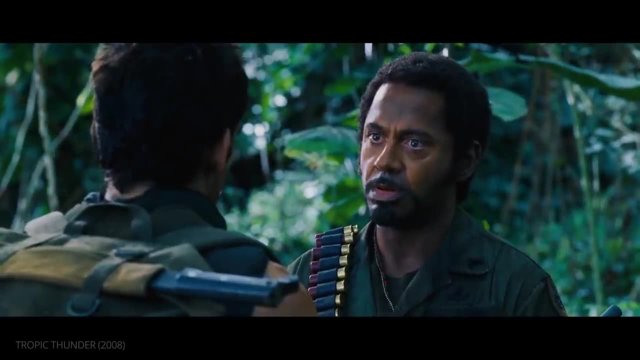 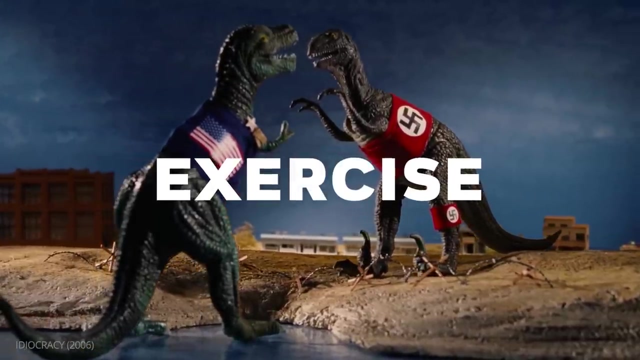 Right, S*** off Hitler". You can probably tell at this point that satire takes many forms. "- You went full retard, man, Never go full retard". But to write an effective satire of any type, here are some steps that can be helpful. 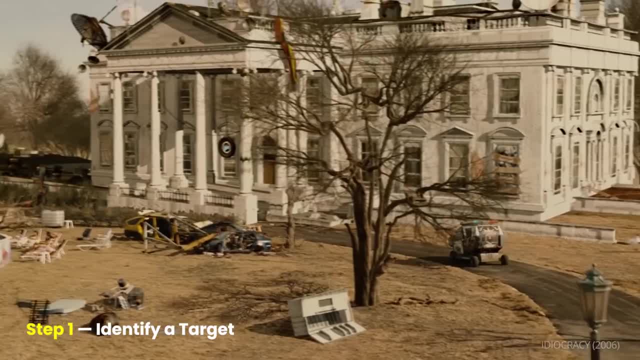 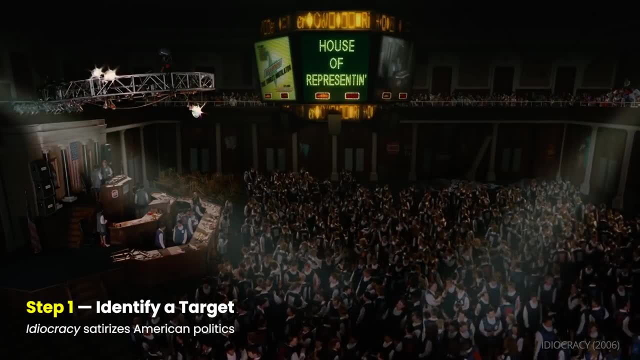 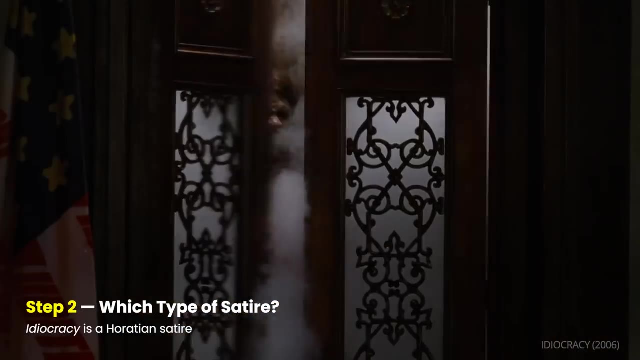 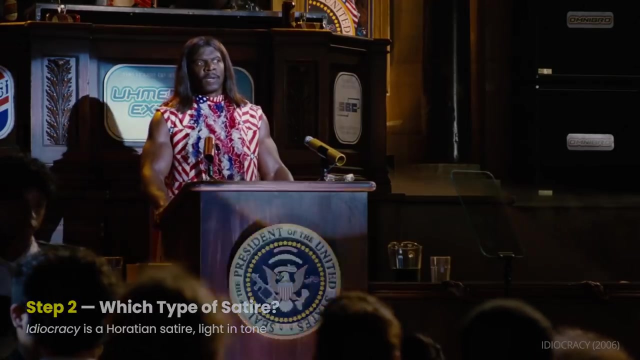 Step one: Identify a target. What system or widely held belief do you think needs changing? Step two: Decide which type of satire would help achieve your goals. "- Ladies and gentlemen, President of America, President Kalanchoe Shut up. 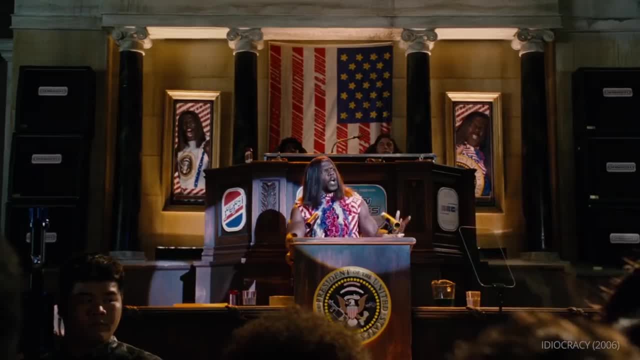 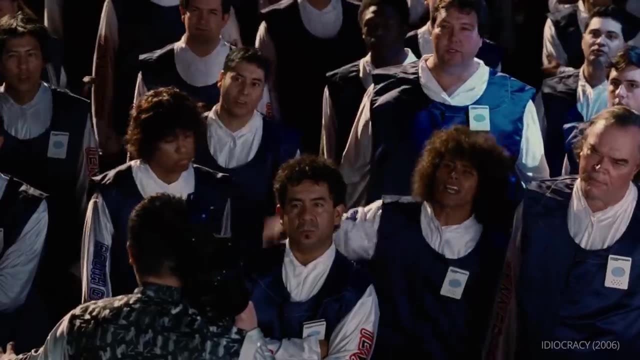 Sit your monkey ass down. I know s*** is bad right now, With all that starving bulls And we running out of french fries and burrito coverings. "- Yeah, But I got a solution. "-. That's what you said last time, dibs. 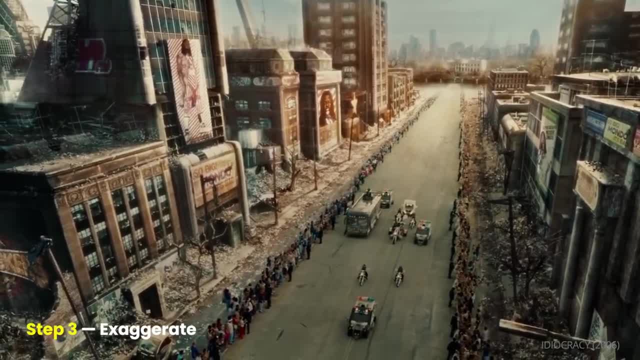 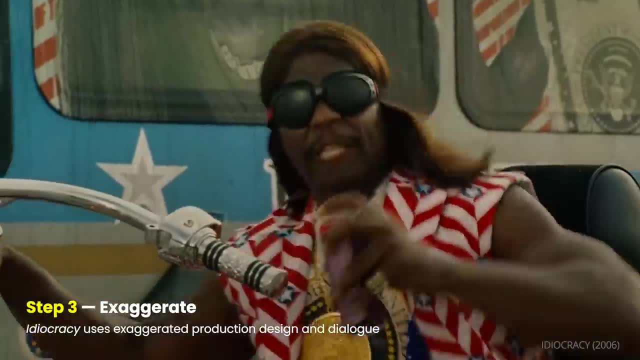 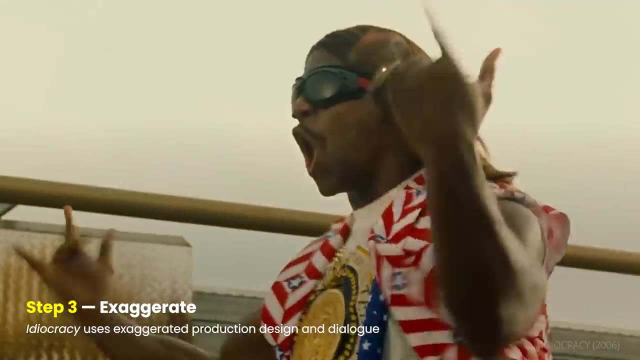 That's what I thought" Step three: Decide how you'll use filmmaking techniques to bring satire into the project. Are there sets or costumes which can be exaggerated? "- Hold on, Vato, Ha-ha, Whoo, Wow, Woo-hoo. 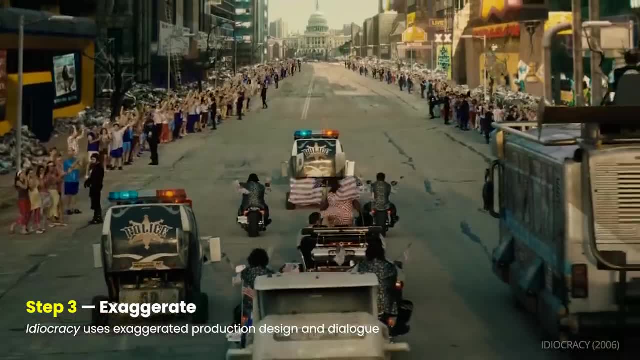 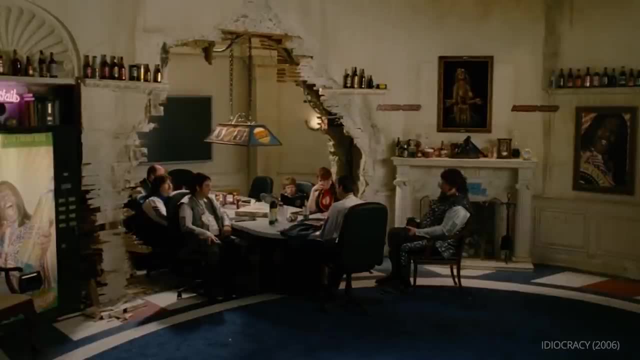 Whoo-hoo, Whoa. Can you inject irony into the dialogue? "- For the last time, I'm pretty sure what's killing the crops is this Brondo stuff "-. But Brondo's got what plants crave: It's got electrolytes. 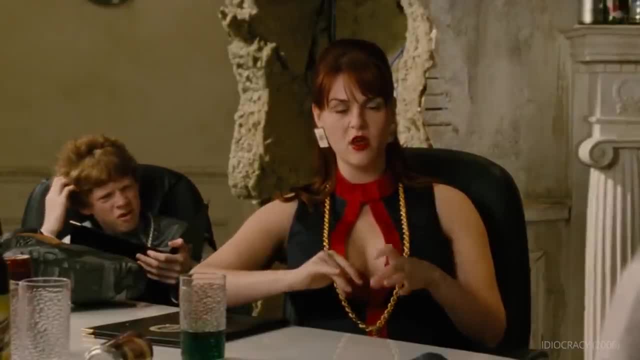 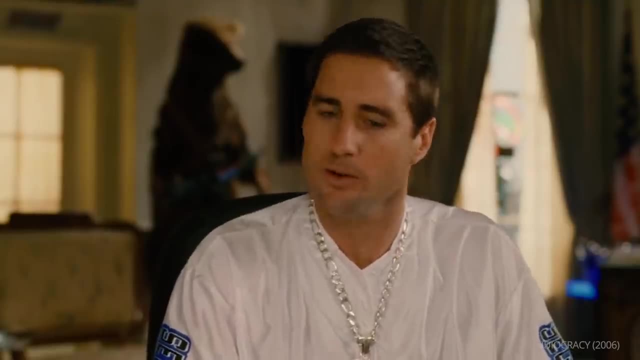 "- So wait a minute. What you're saying is that you want us to put water on the crops. "- Yes, "- Water Like out the toilet "-. Well, I mean, it doesn't have to be out of the toilet, But yeah, that's the idea.